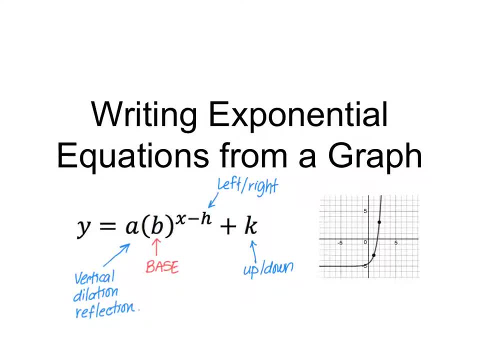 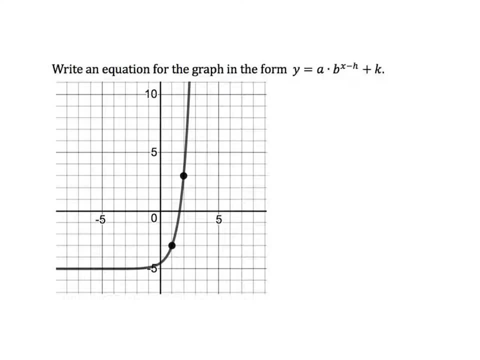 sort of dilation or reflection. With that in mind, let's give a couple examples. a go Okay, in this situation you're given the graph of an exponential function and you're asked to create the equation. So step one is going to be thinking about where's the new? 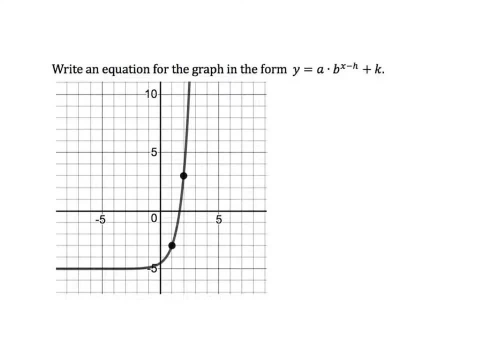 horizontal asymptote. Every exponential function has a horizontal asymptote and the asymptote is the line that the graph gets closer and closer to but never touches. It's normally the x-axis if it's the parent function, but in this case you'll notice that 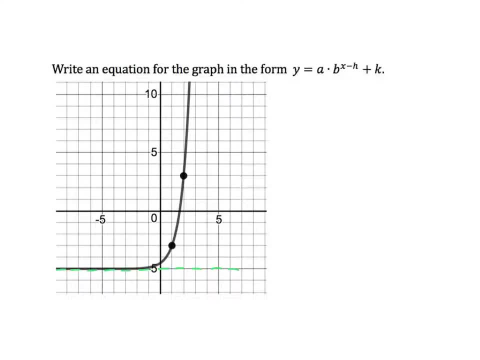 the horizontal asymptote has been shifted down. It's been shifted down five units. So step one: identify your new horizontal asymptote. That's gonna help you determine the k-value in the equation. In this case, we found out that it went down five. The equation of that asymptote would: 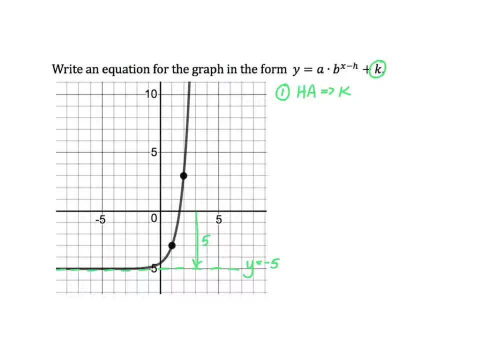 be y equals negative five. So now that we know about the up-down or the vertical, we can try to shift. let's figure out step two. is there a left or right horizontal shift? one great way to do this is to look for an exact point on the graph, probably the 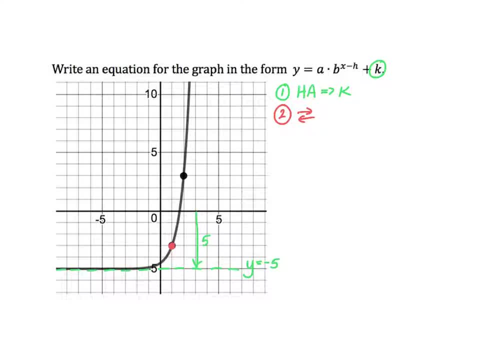 one that's closest to the asymptote, closest in, and consider that as your starting value, and so we can draw a new y-axis right through that point. that'll help us determine the left-right shift. y-axis is normally well at zero, and now it's there, which is one, so we know that we have a shift of one that's going to. 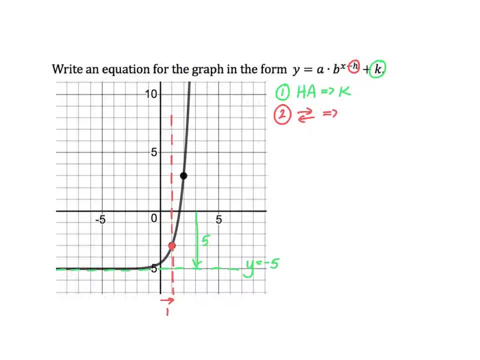 help us with our H value. so now our exponent. since the shift right, we're gonna go X minus one will be our exponent. all right, we've set up our grid, we know our horizontal and vertical translations. next step is to figure out the a value, that last transformation in the equation. so the best way to figure. 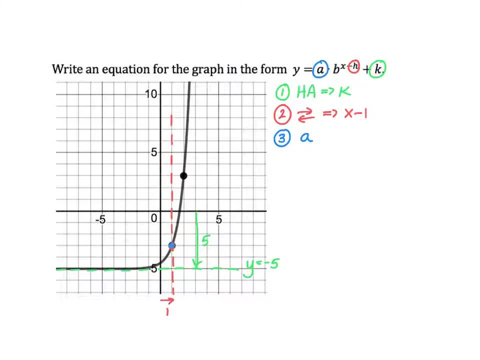 out. the a value is to go back to that closest point that you drew, to the asymptote. consider that point, count how many units that is away from the asymptote, and in this case it's two. that's going to represent your a value. now that you're here, let's set up the. 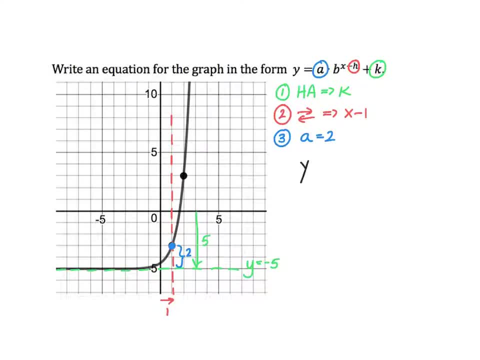 equation, including all those transformations that we found so far. so y equals a is 2 B. we still don't know. we know it's growth, so it's going to be bigger than one, but we don't have it just yet. shift to the right. so X minus. 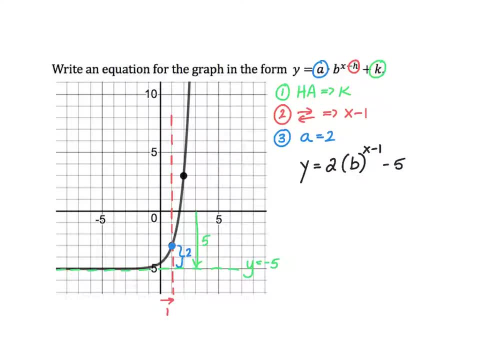 one shift down, so minus five. last step is to figure out what is the value of the B. what is the B value? so you want to choose a different point than you've used so far? let's use this one. they give it up to us nicely, it's. 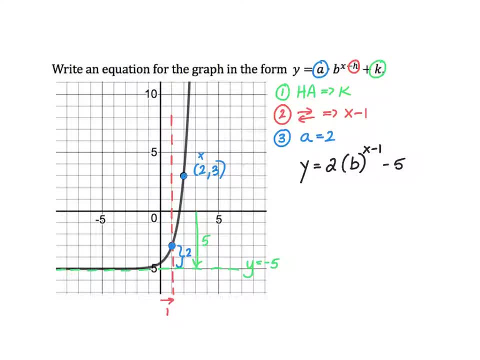 the point two, three, so you can plug X is two into the equation and Y is three into the equation and use that to solve for B. so let's do that: plugging in three for Y, leaving B as it is, plugging in two for X and solving. make sure you follow. 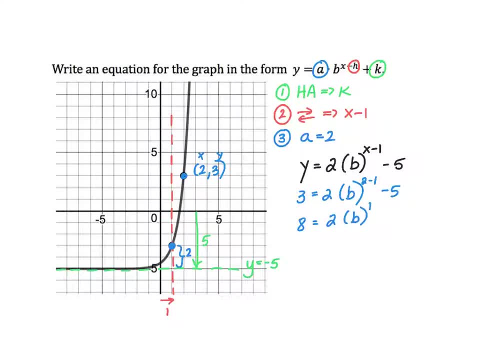 the correct order of operations as you go about this, dividing both sides by two, so I get: four is B or B is four. there we go, we notice that your B value is bigger than one, which you would expect, because this is growth. as X values get bigger in this end behavior, Y values are also getting bigger, so this is showing. 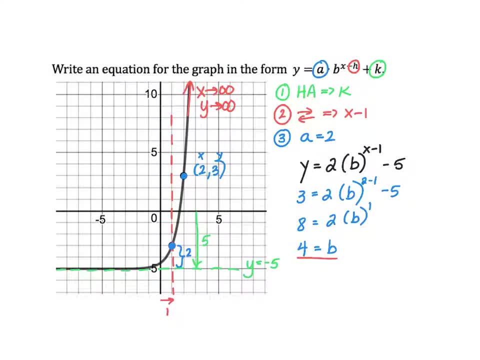 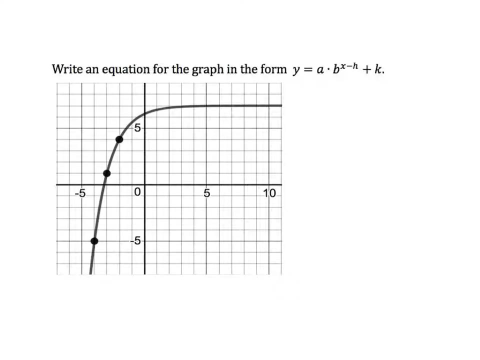 its growth. our B value of four confirms that that's growth. so final answer here: Y equals two times four to the X minus one minus five. here's another example of an exponential graph and we're asked to create the equation. so if we want to do that, let's. 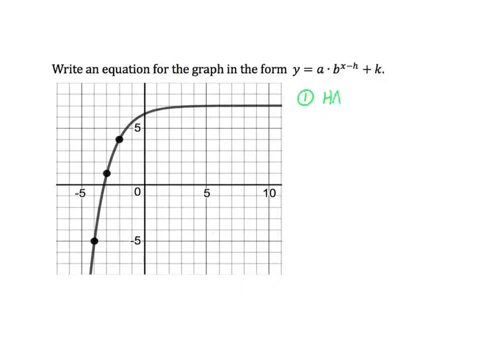 start with step one, which is identifying the horizontal asymptote. the parent function would have an asymptote at zero. this one has an asymptote all the way up at six, which means we have a vertical shift of six. that tells us that the K value in the equation will be six. now that we know the up-down shift, let's 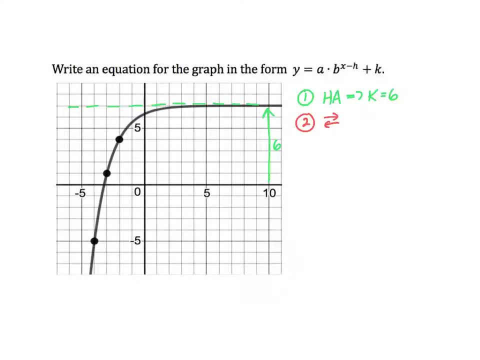 look for a left-right shift so find a point that is closest to the asymptote, an exact point. there it is. now let's look for a left-right shift, so find a point that is right there and put a new y-axis through there. now we can see that we. 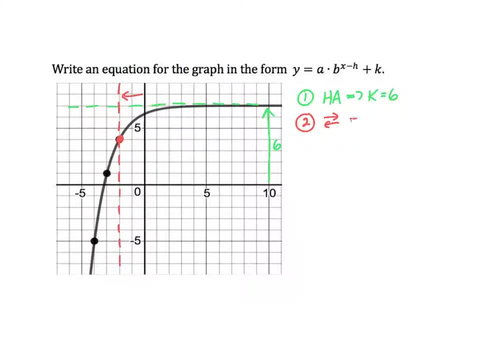 have a shift left by two. so a shift left by two means in your equation you're gonna have an X plus two as your exponent. the last transformation we need to determine is the a value. so go back to that closest point. count how many points it is away from the asymptote. in this case it's three points away. but